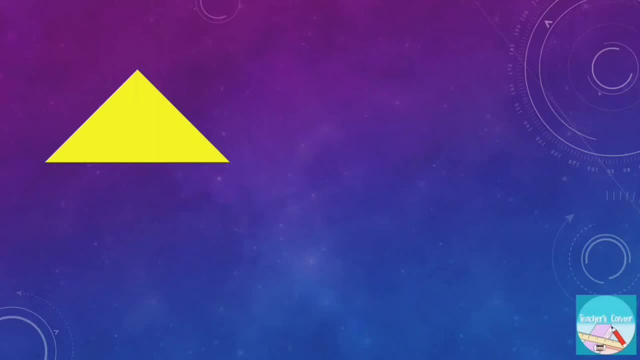 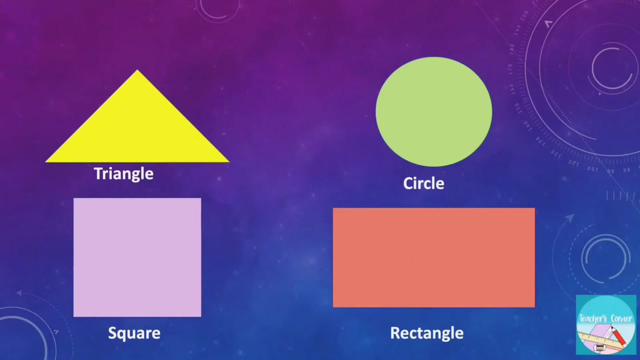 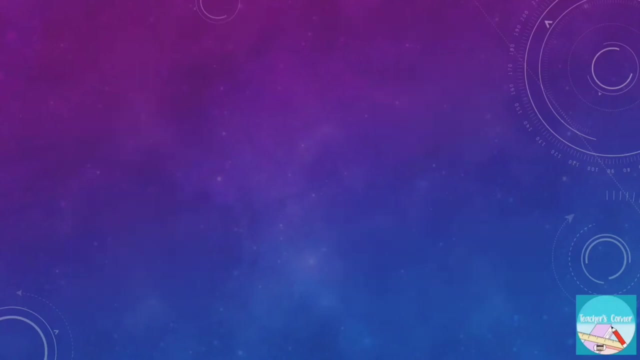 What is this? This is a triangle. What is this? This is a circle. Now see this. This is a square. This is a rectangle. Now tell me, what type of geometrical shapes are these? Yes, These are plain geometrical shapes. Now see some more shapes. What is this? This? 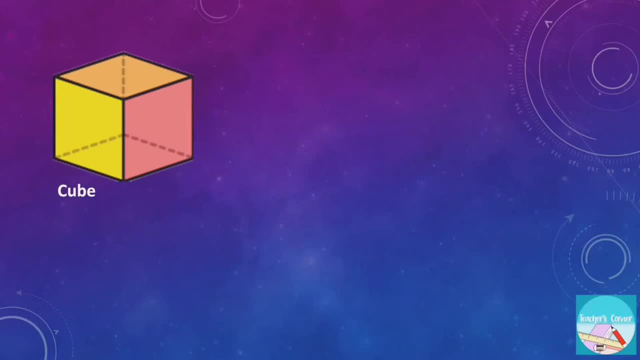 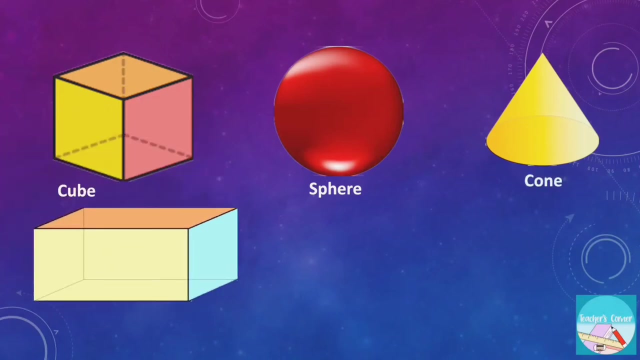 is a cube. This is a jumping sphere. This is a cone. This is a cone. This is a ball. What is this? This is a ball. What is this? This is a ball. What is this? This is a ball. 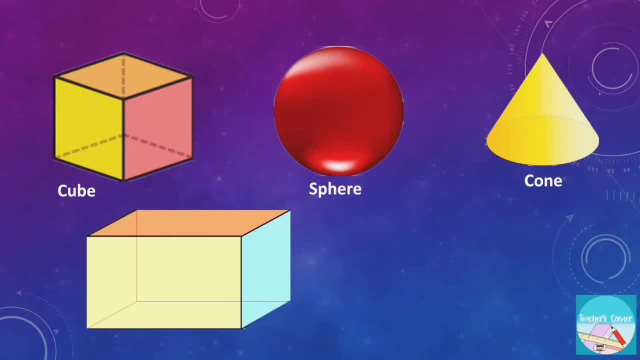 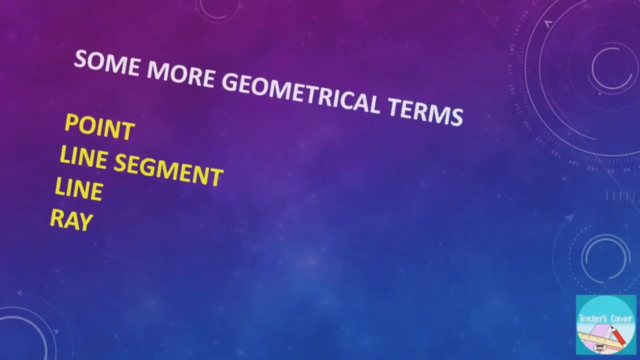 Now see, this is a cuboid, this is a cylinder. very good, Now tell me what type of geometrical shapes are these? yes, these are solid geometrical shapes. Now, children, in this video, we are going to learn about some more geometrical terms that. 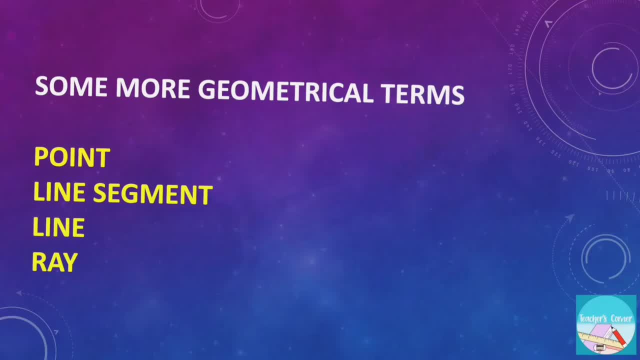 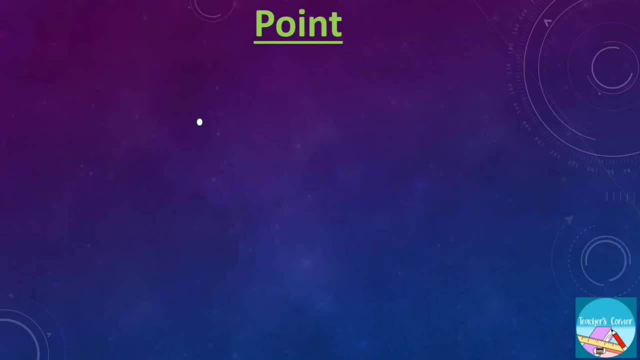 is point line, segment line and ray point. These are some points. a point is represented by a small dot. It is very small in size, like a tip of a pencil or a tip of a pen. We write the name of the points by using a pen. 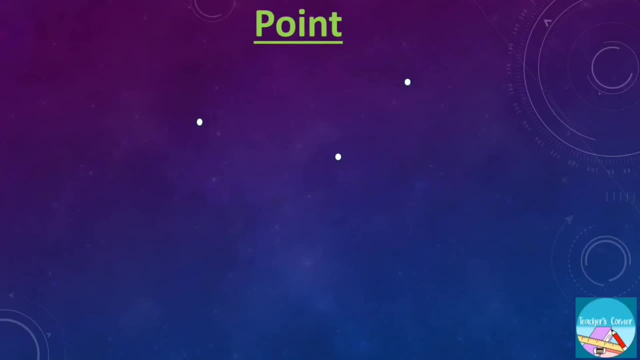 Using some alphabetical letters. Let us see the name of this point. is point A, point B, point P. In this way, we can write the name of point by writing any capital letter. So what we have learnt here: A point is represented by a small dot. 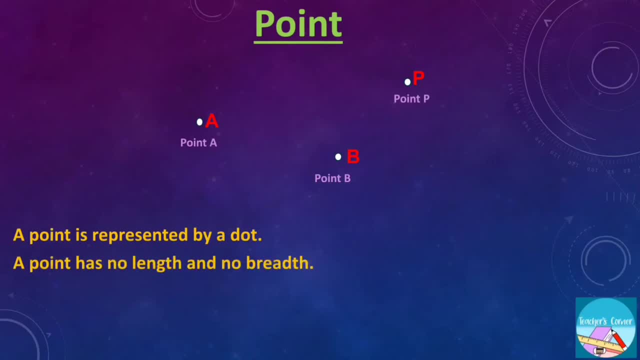 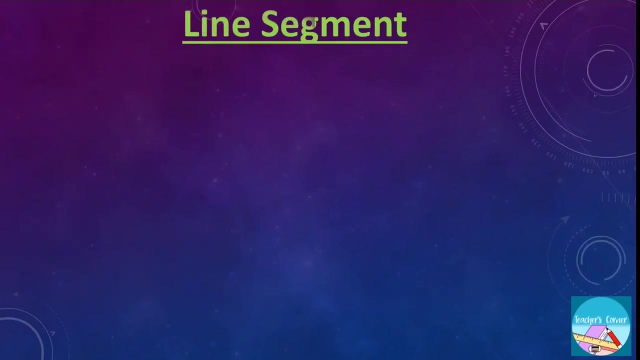 A point has no length and no breadth because it is very small in size. The name of point is written by using any capital letter, like A, B, P, X, Y, Z, etc. Line segment. Here we have two points: A, B, P, X, Y, Z, etc. 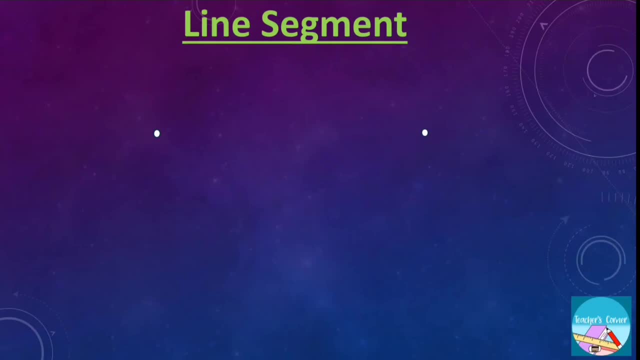 Line segment. Here we have two points. When we join these two points, point A and point B, we get a line segment A- B. When we write the name of a line segment, we always write a bar over it. A line segment has two end points, point A and point B, So it has a fixed length. 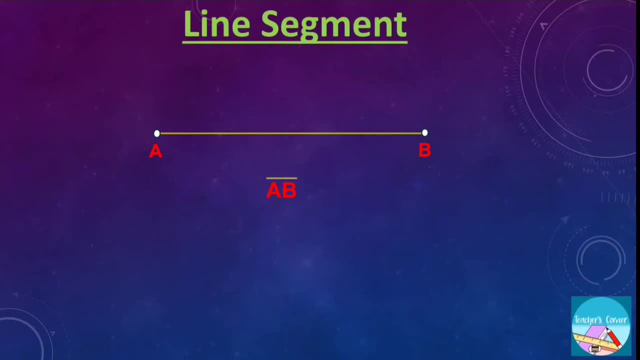 Now see what we have learnt. Now see what we have learnt. A: B is a line segment. When we join two points, we get a line segment. A line segment has two end points, So it has a fixed length. 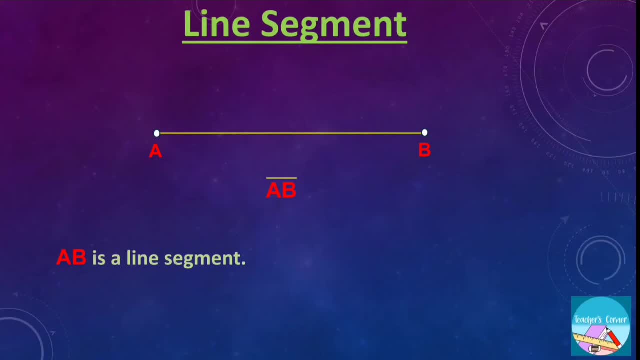 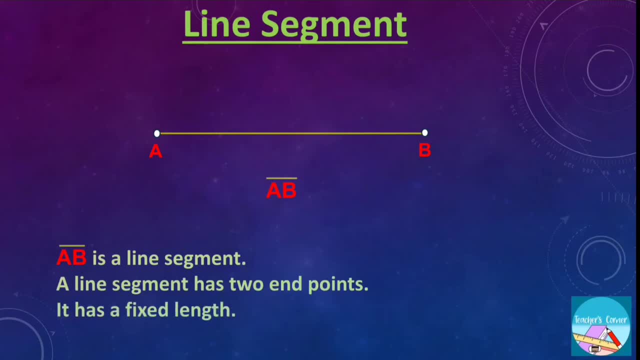 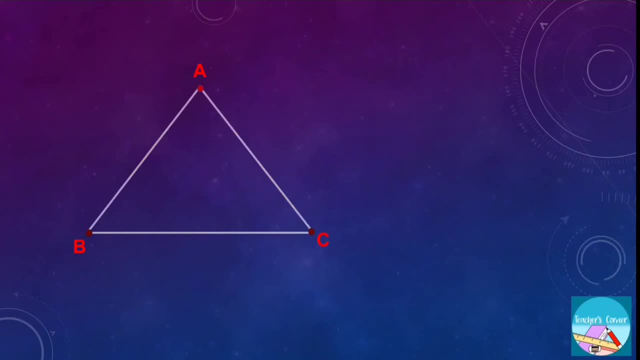 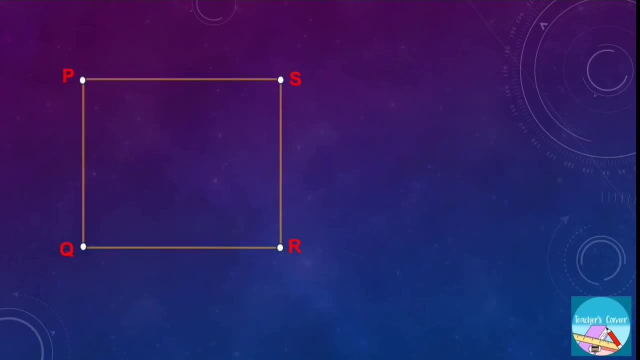 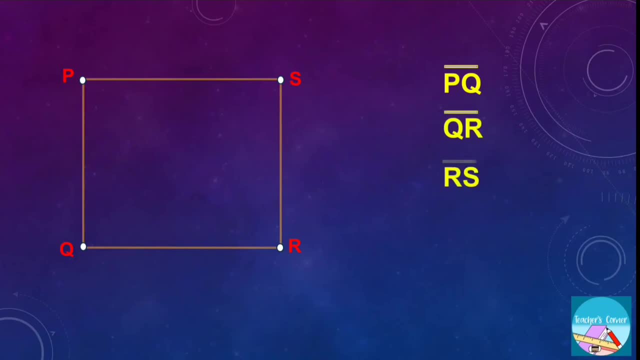 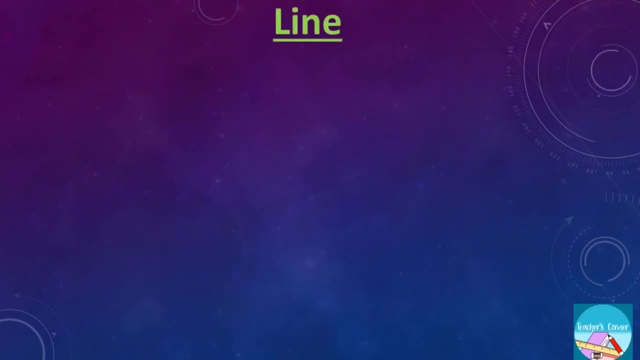 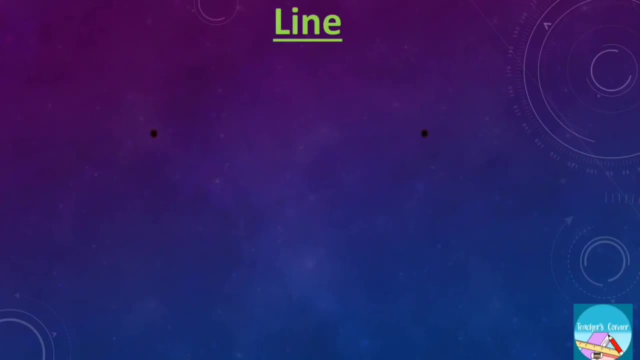 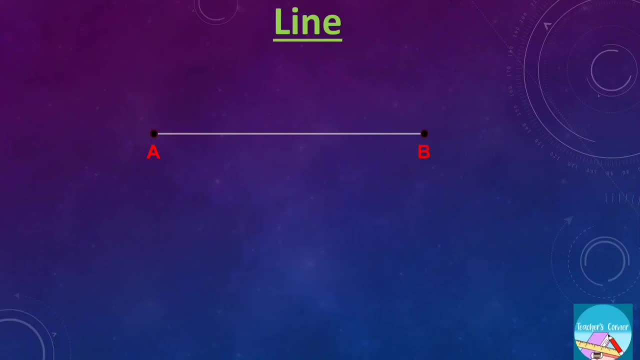 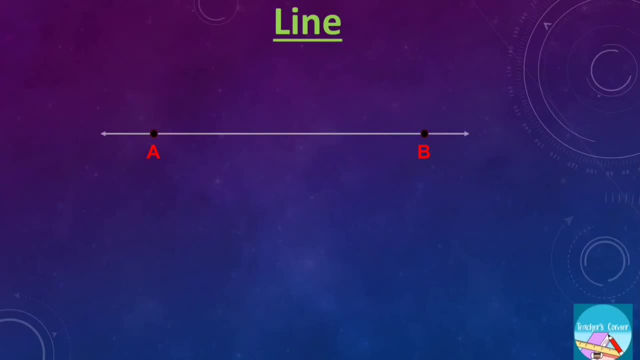 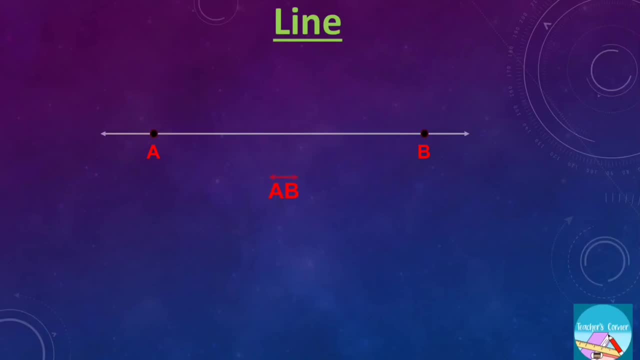 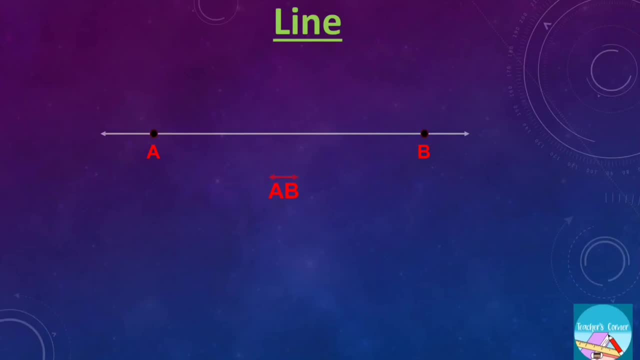 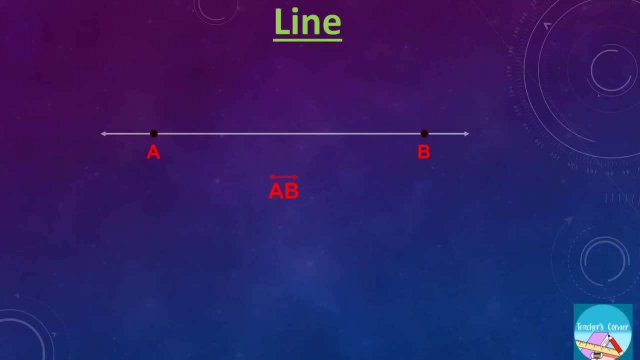 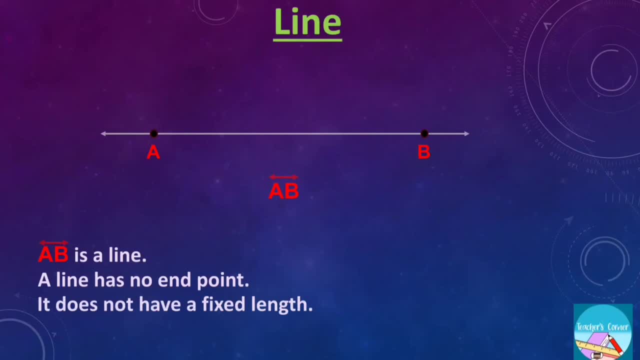 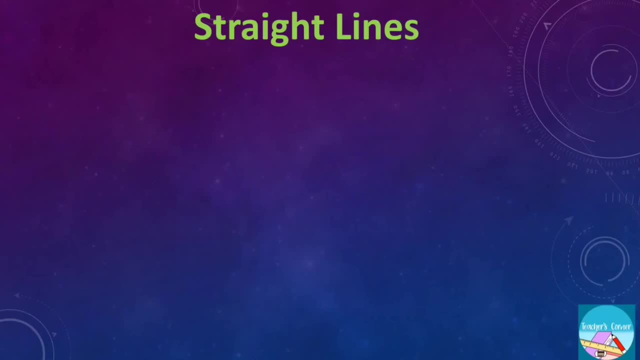 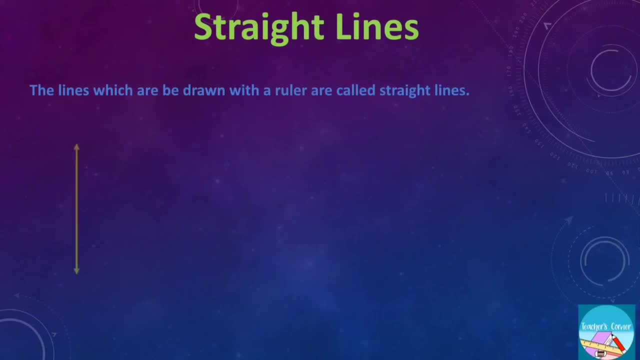 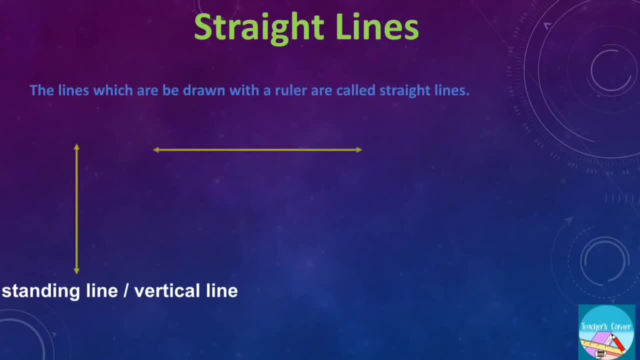 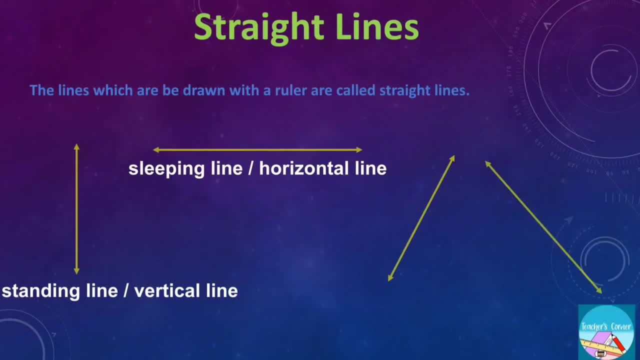 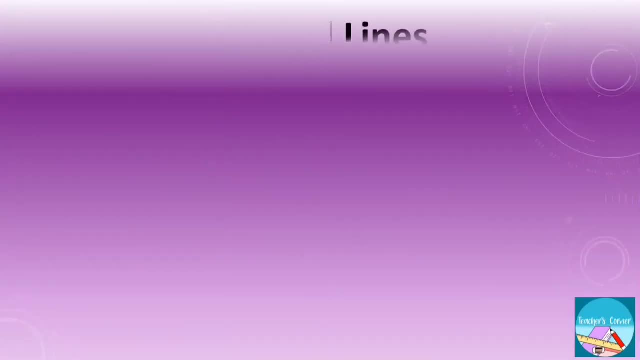 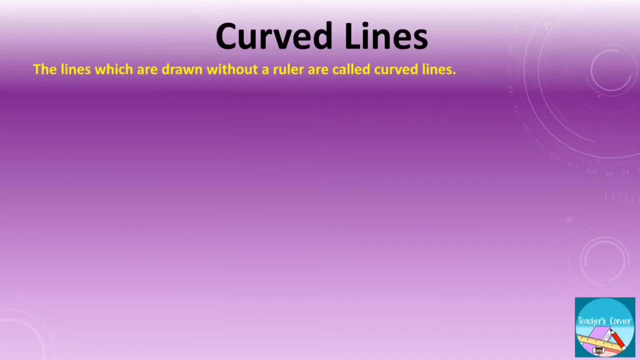 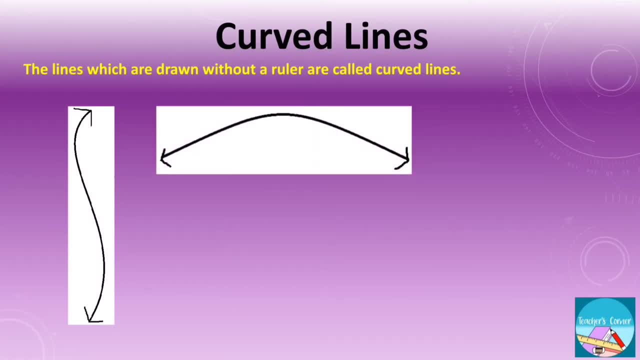 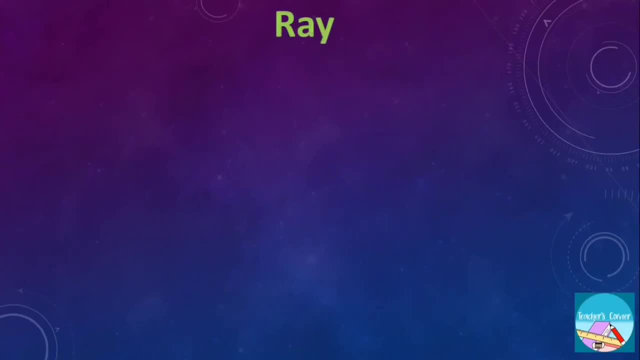 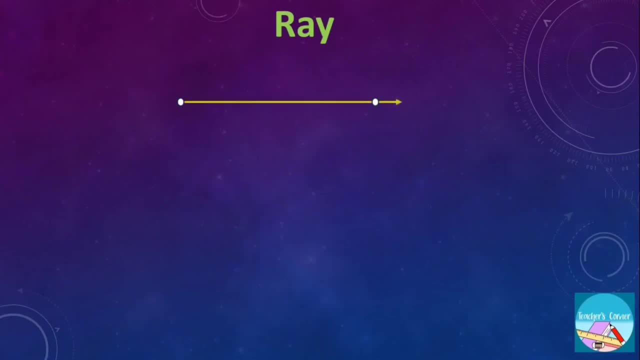 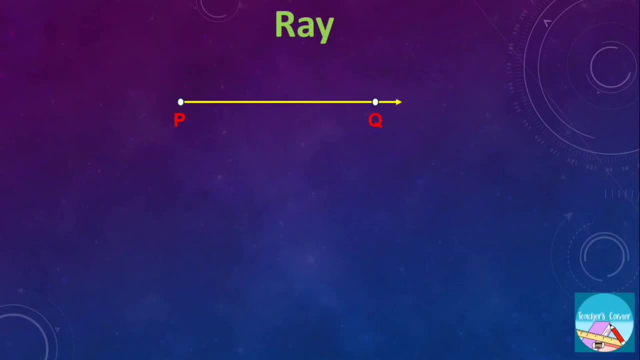 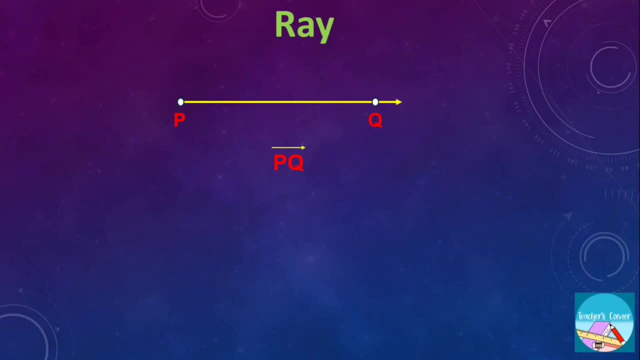 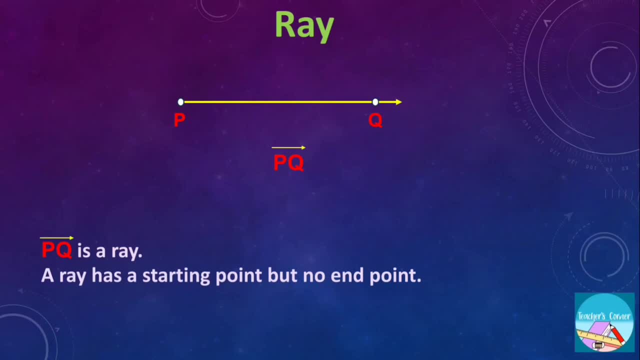 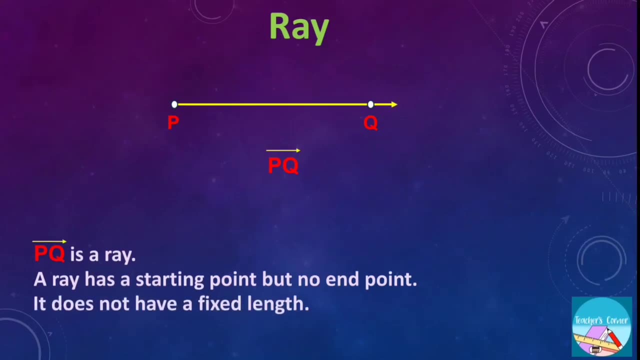 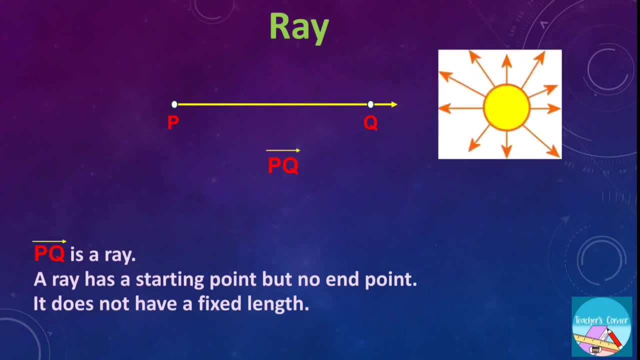 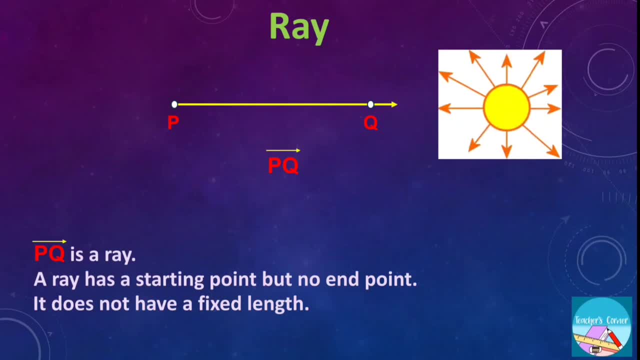 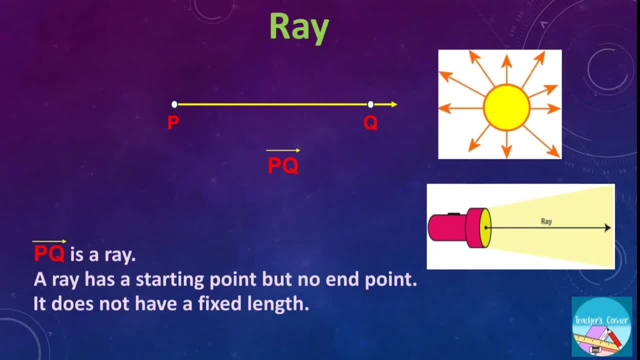 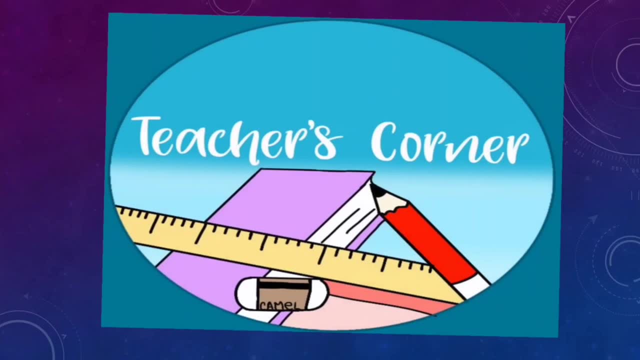 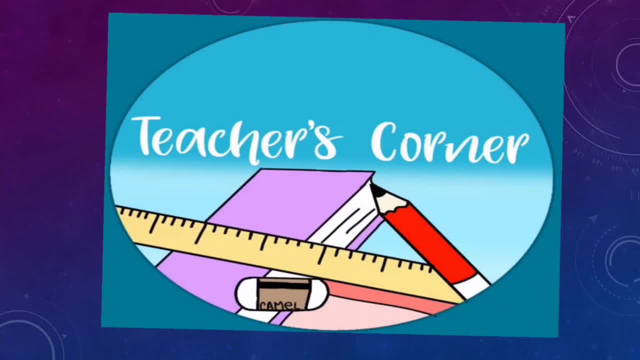 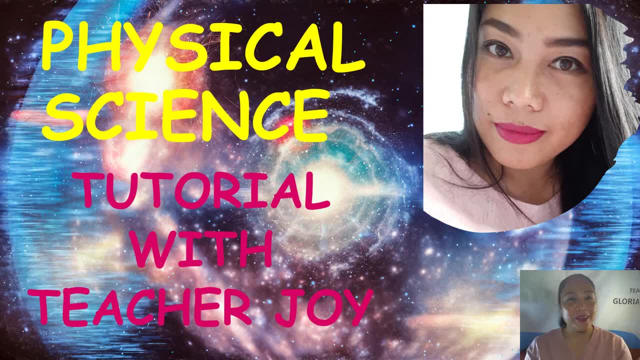 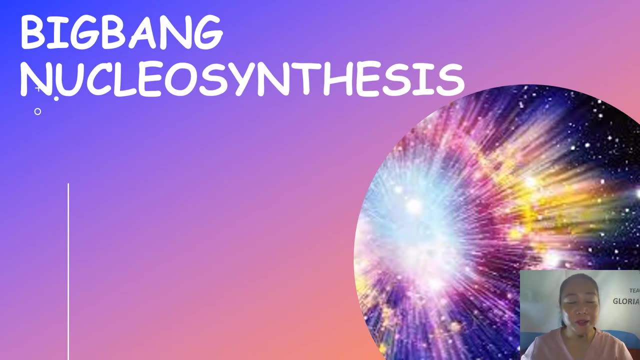 Hello everyone, Welcome back to another video lesson with me, Teacher Joy. In today's tutorial we will have physical science. Let's discuss about Big Bang, Nucleosynthesis, the beginning of elements, the formation of the light elements in the Big Bang Theory.